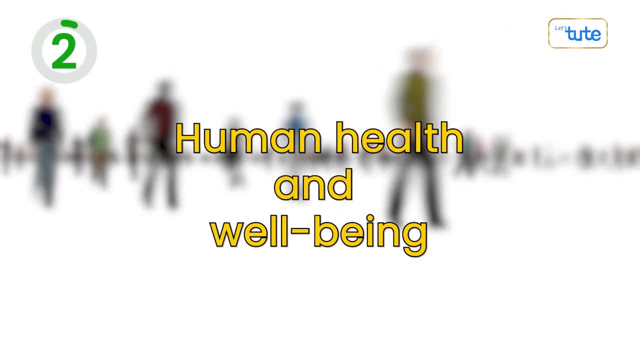 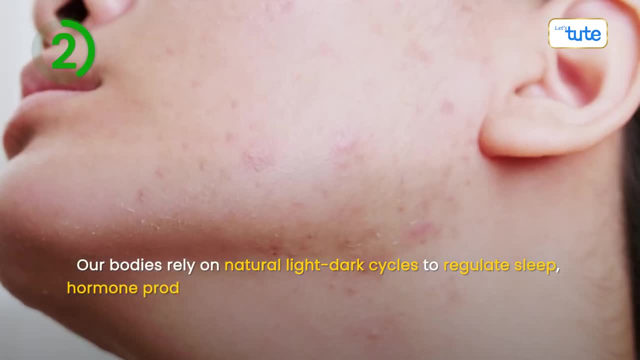 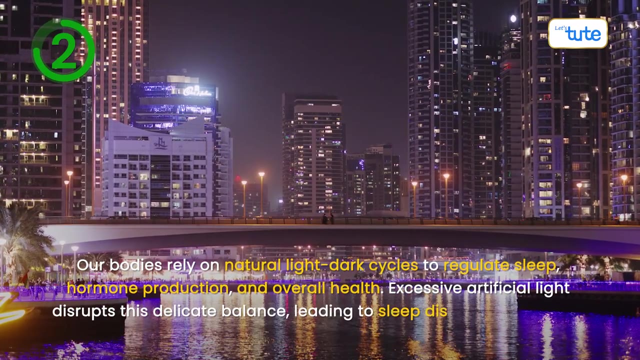 the birds that migrate at night. Light pollution affects human health and well-being. Our bodies rely on natural light-dark cycles to regulate sleep, hormone production and overall health. Excessive artificial light disrupts this delicate balance, leading to sleep disorders, anxiety. 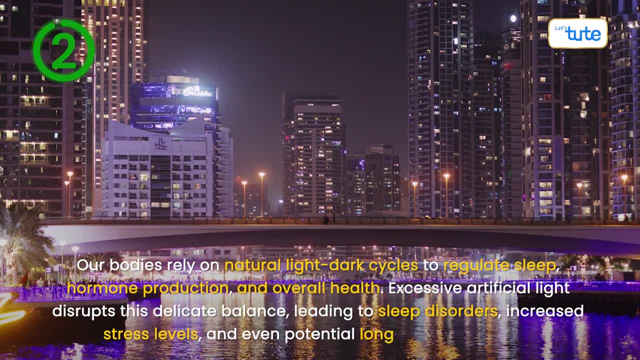 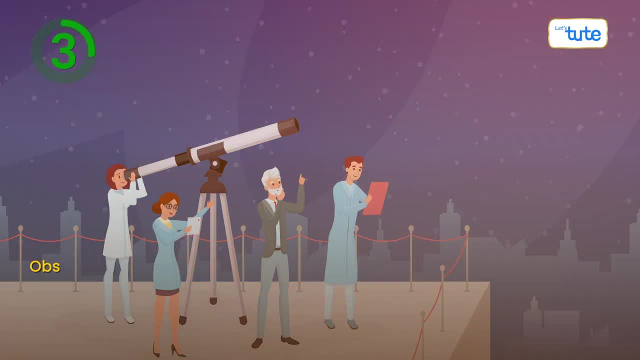 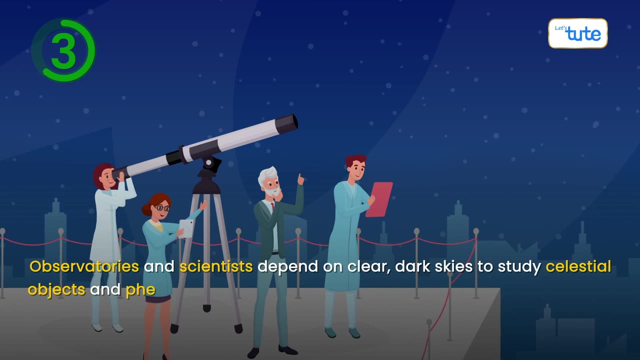 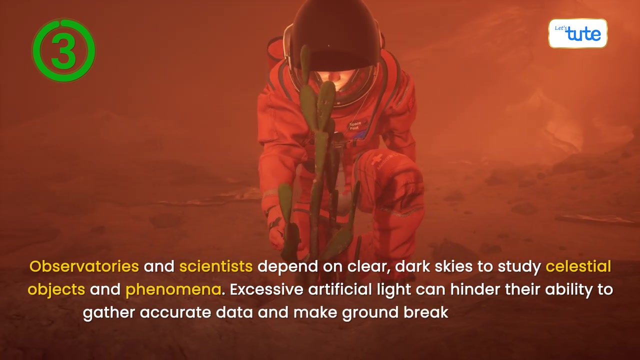 depression, increased stress levels and even the potential long-term health risks. Light pollution can impact astronomical research and observations. Observatories and scientists depend on clear, dark skies to study celestial objects and phenomena. Excessive artificial light can hinder the ability to gather accurate data and make groundbreaking discoveries. 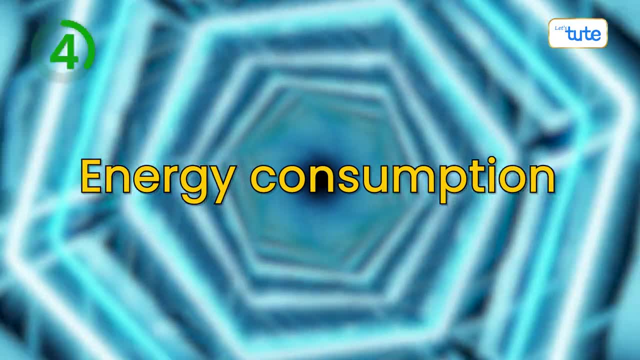 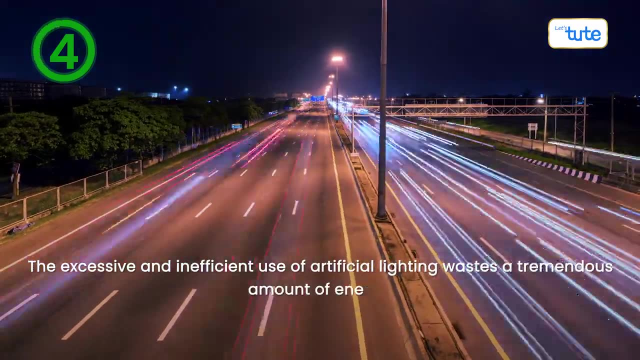 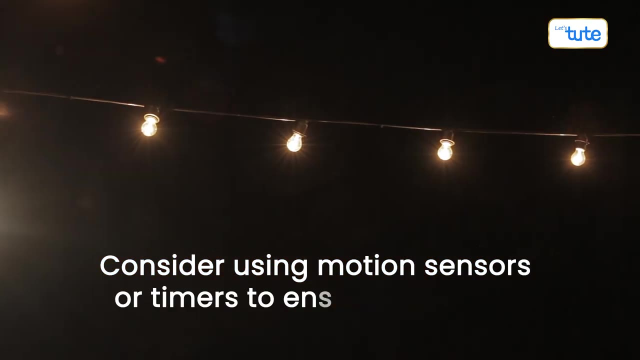 Light pollution also has a significant impact on energy consumption. The excessive and inefficient use of artificial lighting wastes a tremendous amount of energy. How can we reduce this pollution? Firstly, we can start by using outdoor lighting responsibly. Consider using motion sensors or timers to ensure lights are only active. 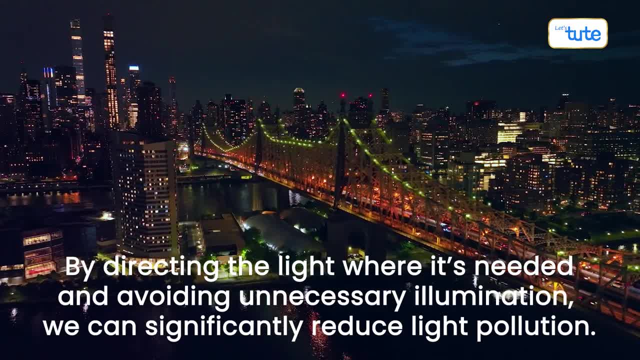 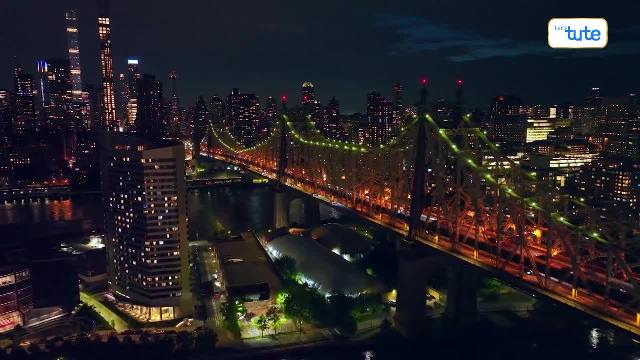 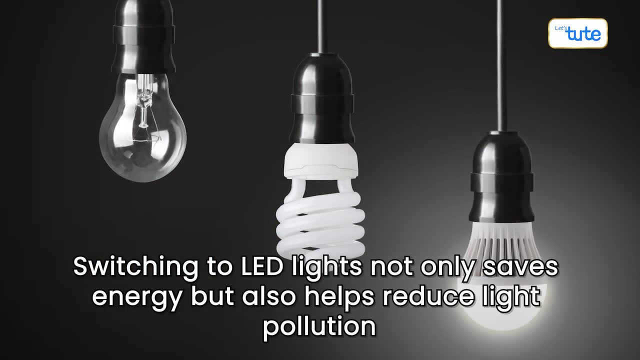 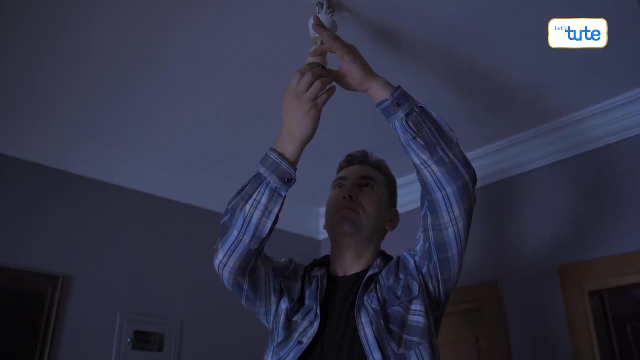 or needed. By directing the light where it's needed and avoiding unnecessary illumination, we can significantly reduce light pollution. Reduce the use of decorative lighting. Let's prioritize energy-efficient lighting options. Switching to LED lights not only saves energy, but also helps reduce light pollution. Thus, by making small changes in our own lives and 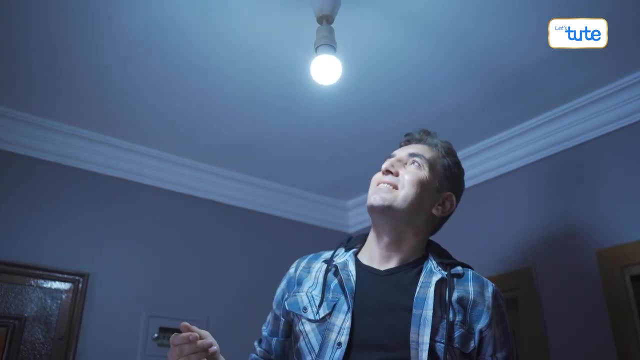 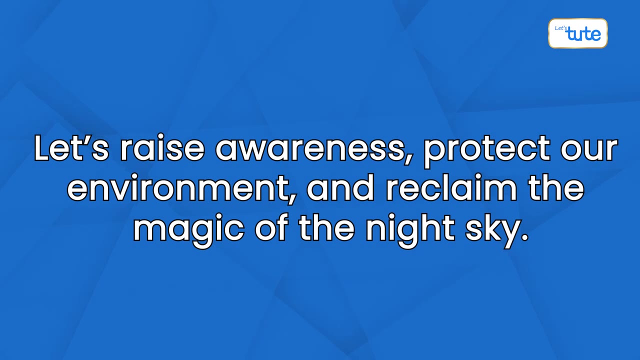 advocating responsible lighting practices, we can make a tangible difference. Together, let's raise awareness, protect our environment and reclaim the magic of the night sky. That's it for today. Hope the video was informative. Thanks for watching. If you liked the video, hit the like button and please share it with your family and friends. 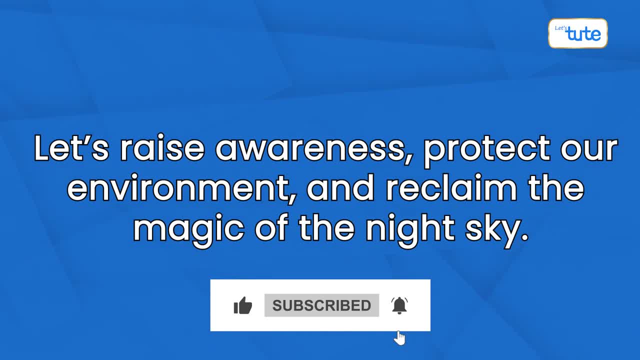 to spread awareness. Subscribe to our channel for more. Thank you for watching.